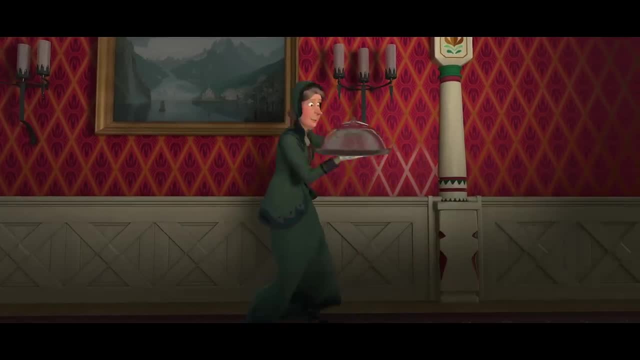 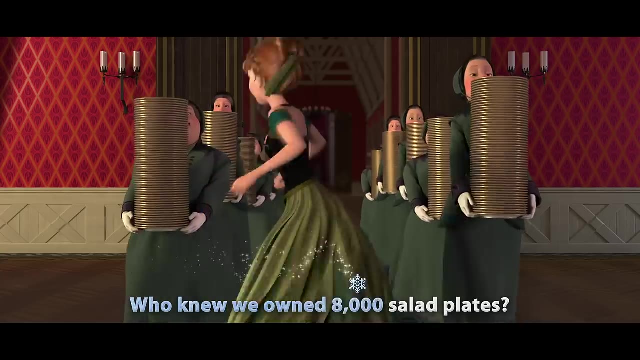 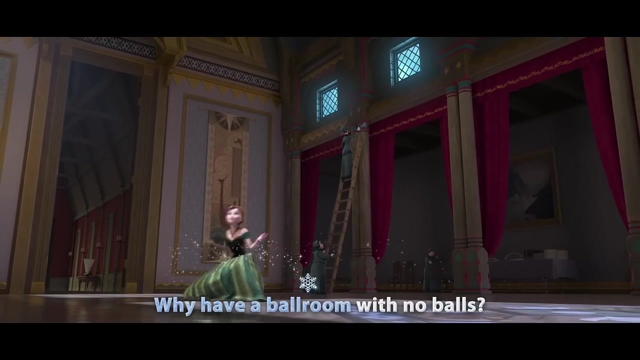 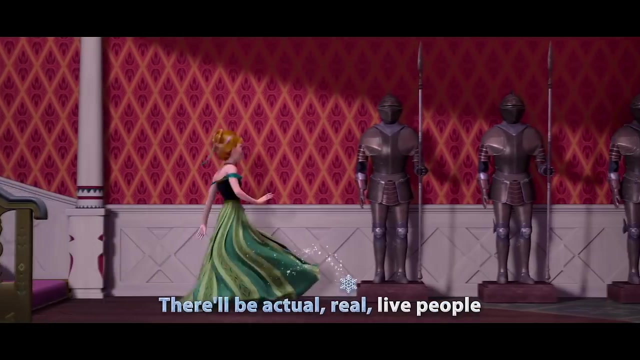 The window is open, so's that door. I didn't know they did that anymore. Who knew? we owned 8,000 salad plates. For years I've roamed these empty halls. Why have a ballroom with no balls? Finally they're opening up the gates. They'll be actual, real life people. It'll 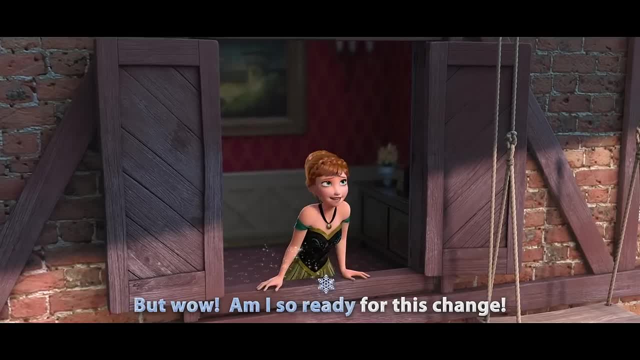 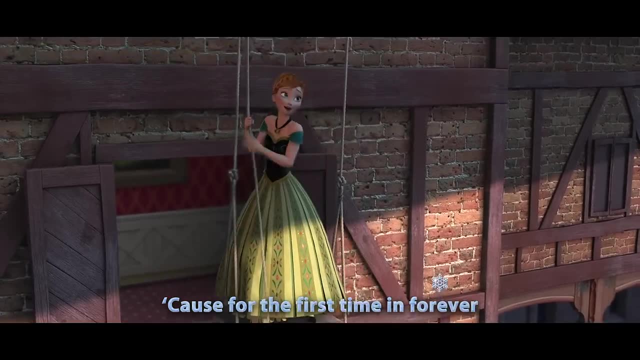 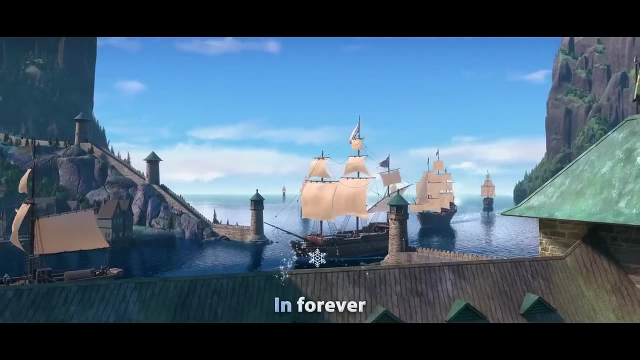 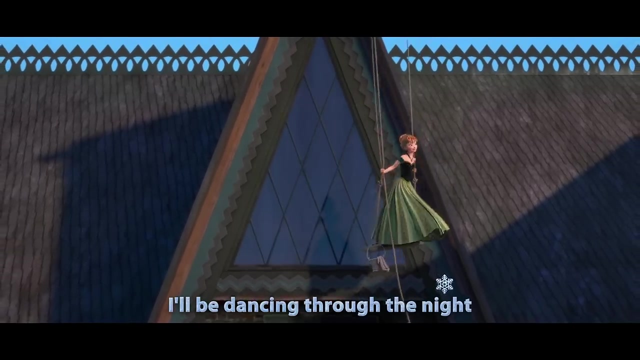 be totally strange. But, wow, am I so ready for this change? Cause, for the first time in forever, there'll be music, there'll be light. For the first time in forever, I'll be dancing through the night. Don't know if I'm elated or gassy, but I'm somewhere in. 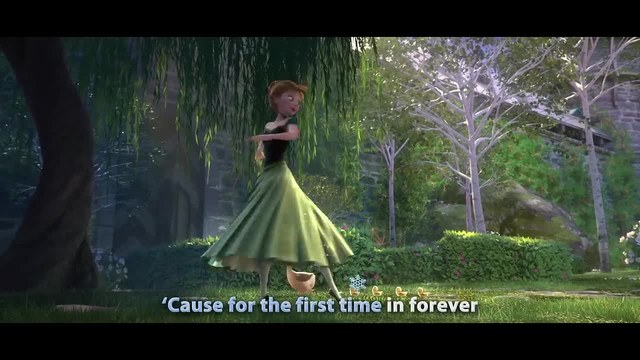 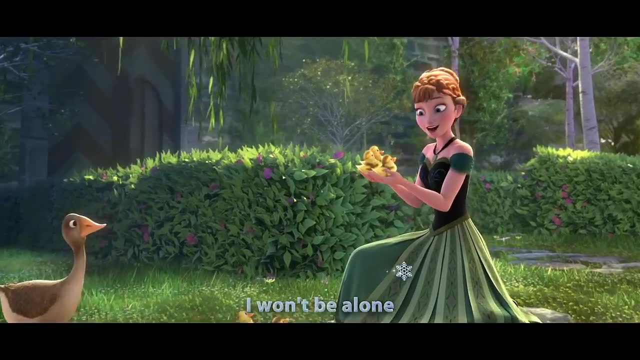 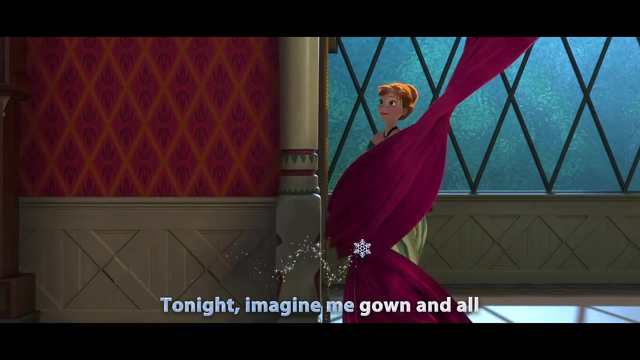 that zone, Cause, for the first time in forever, I won't be alone. I can't wait to meet everyone. What if I meet the one Tonight? imagine me gown and all fetchingly draped against the wall, The picture of sophisticated 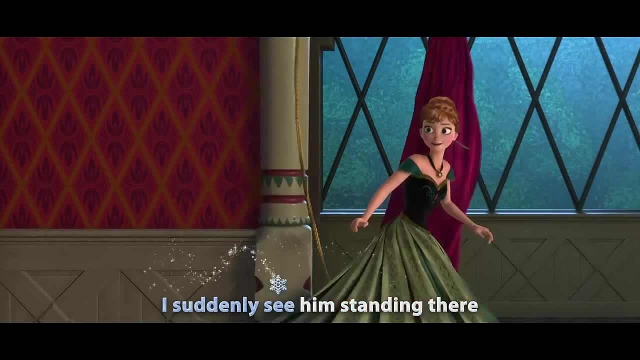 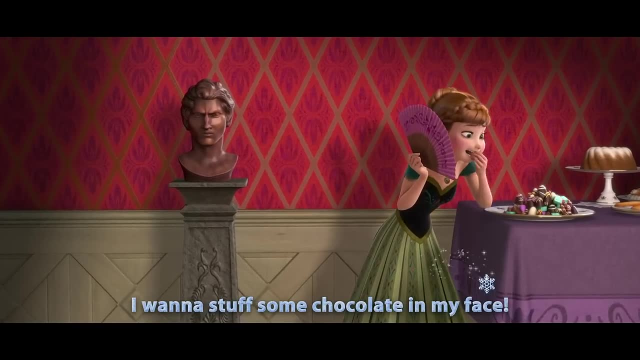 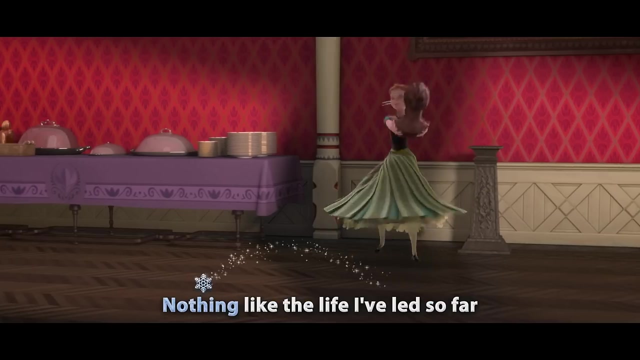 grace. I suddenly see him standing there, a beautiful stranger, tall and fair. I want to suffocate. Some jog would hurt my face. But then we laugh and talk all evening, which is totally bizarre. Nothing like the life I've led so far. 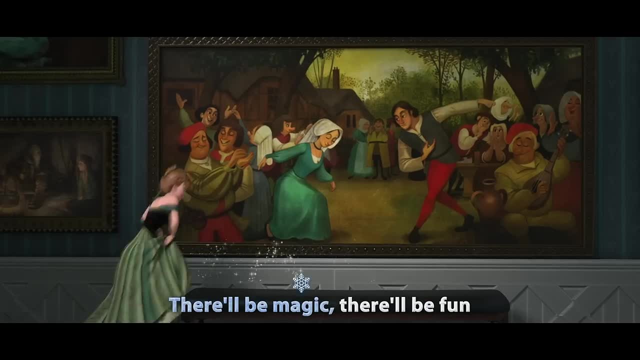 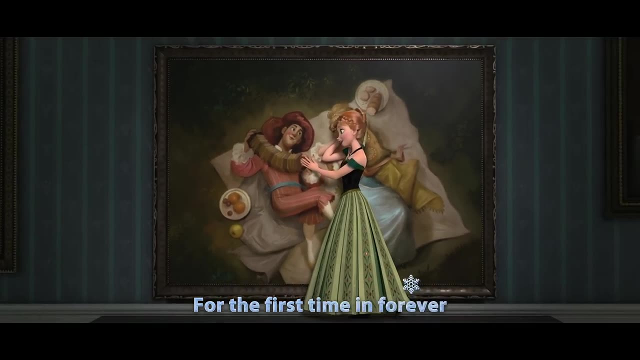 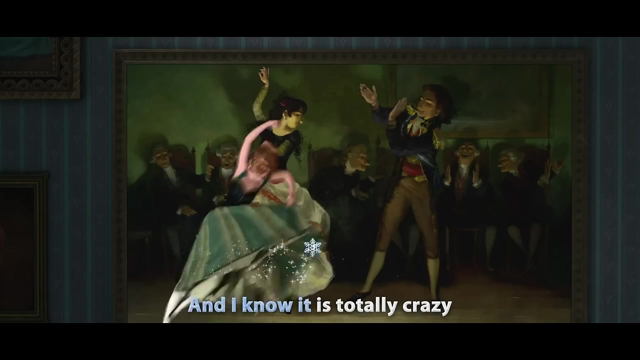 For the first time in forever there'll be magic, there'll be fun. For the first time in forever I could be noticed by someone- And I know it is totally crazy to dream I'd find romance. But for the first time in forever…. 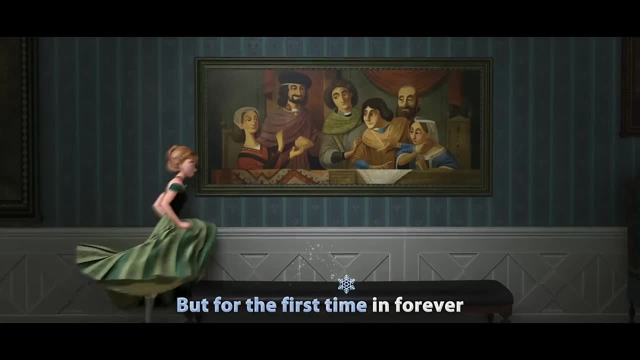 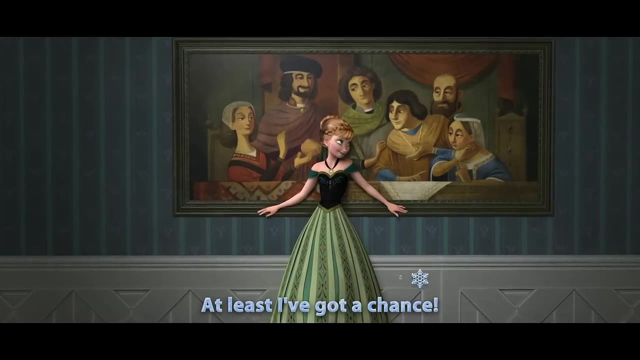 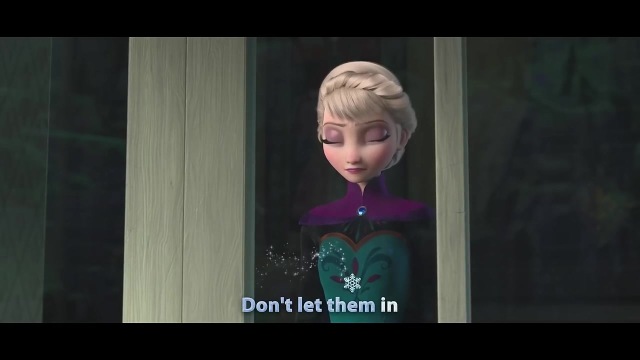 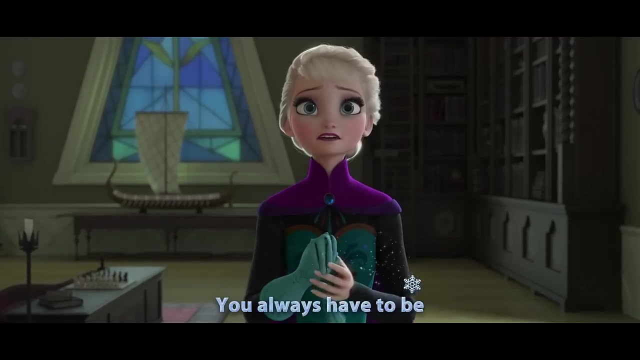 At least I've got a chance. Don't let them in, Don't let them see. Be the good girl you always say: Don't let them in, Don't, let them see, Don't let them see who she is have to be.